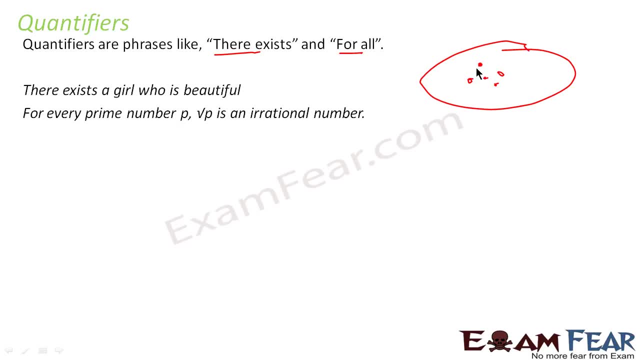 in the school. some are short, summer tall. there is a teacher who has to stop or their exists. a teacher was a big car. Some kids may have small cars, some kids may have big car. So when you're seeing there exists, that means from a bigger set. 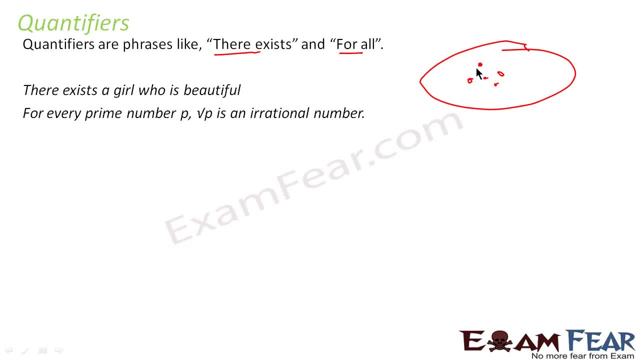 you have at least one, at least one teacher who has big car, or at least one girl who is beautiful. Correct When I say they'll exist a politician who is not corrupt. So that means in our country there are so many politicians, there should be one politician who is non-corrupt. well, actually. 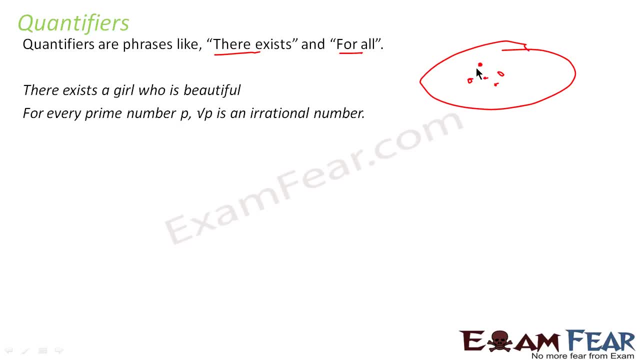 i doubt the statement. but there should be one politician who is non-corrupt. such kind of scenarios we represent, using statement there exist, there exist. and then stick when you say for every, that means for every prime number. if you see p, root, root, p is a rational. 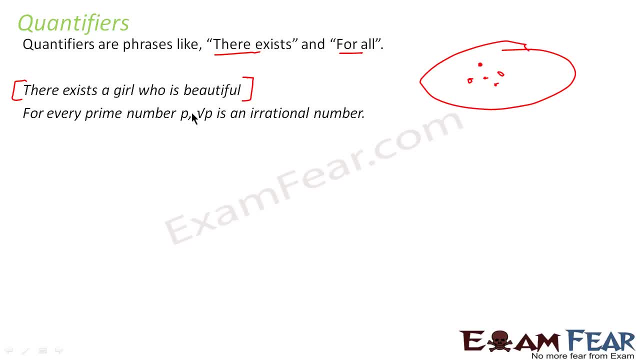 number. so you take any prime number, you take root of the right number. it becomes irrational. so for every is used when the statement is true, for all the elements in the statement. for example, this is again a bigger set and you have element one, two, three, four, five, six, seven, eight, nine, ten. 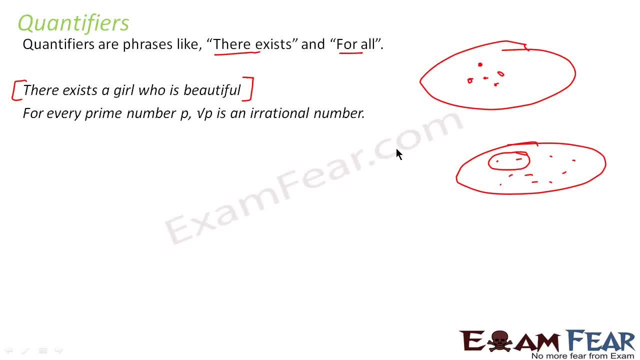 so if your statement is true only for- let's suppose- these statements, then you say there exists. but if your statement is true for all the elements in the set, then you use for every. so if i say for every school there are students, for every school there are students, 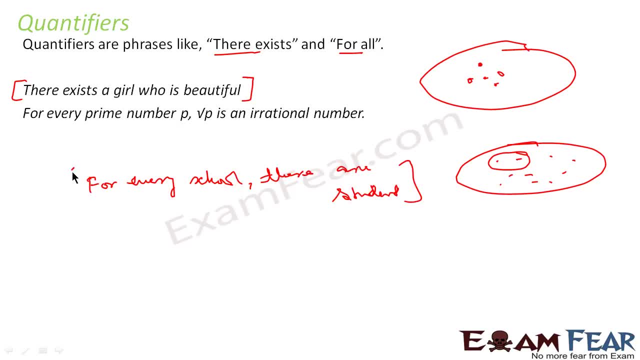 the statement is true because you take any school, there has to be a student. if there is no student, there is no, there is no school. but if i say a statement like this, there exists a teacher in school. let's suppose in school, in my school, i say: 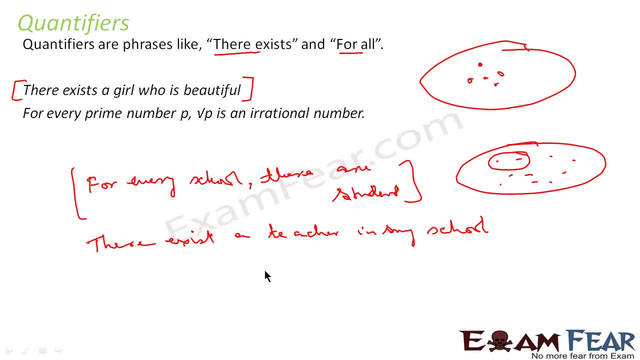 in my school, or in your school and my school, who teach maths. so if you see in your school there are so many teachers but only few of them teach maths, right, so you can say there exists a teacher in your school who teach math. you can't say that for every teacher in your school. the teacher is. 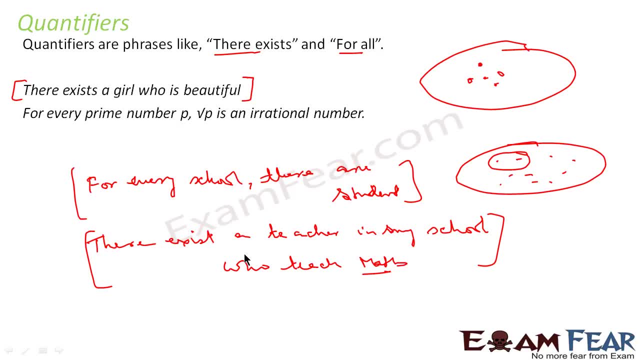 man, because it's not the correct statement. there's some teacher teach math, some teacher may not teach teach math, but for every school there is a student. so i think the concept is clear. when you're saying there exists and then say statement, that means you have a bigger statement, or in your statement. 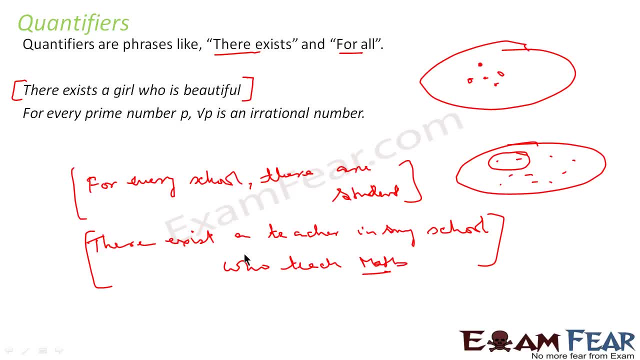 some of the points are true, or some elements are true. when you say for every, then in your set all the elements are true and i say for every school there are students, then every school has a student. and i say there exists a teacher in my school who teach math, that means out of all the. 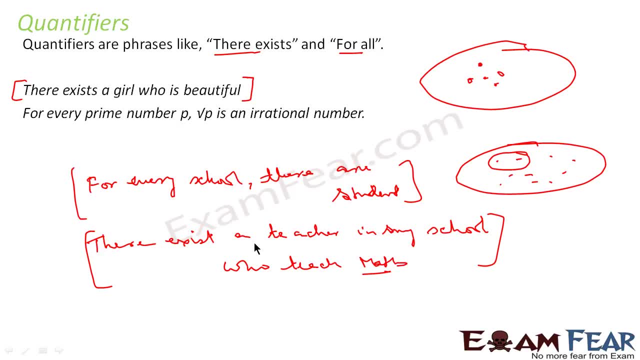 teachers. there are some teachers who teach math, some teachers don't teach math. and i'll say: for every two positive numbers, some is positive. so if you take any two positive number, if you add it, this becomes positive, correct. so you take any two number you add, it becomes positive, so you. 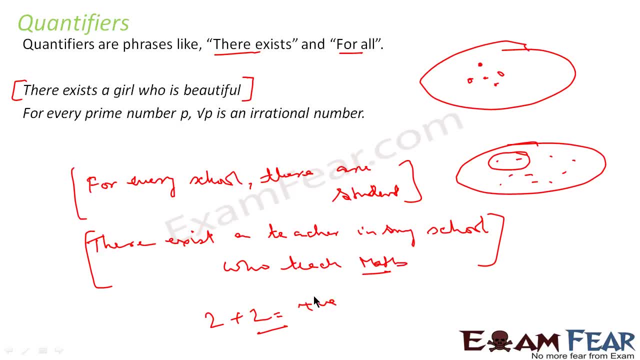 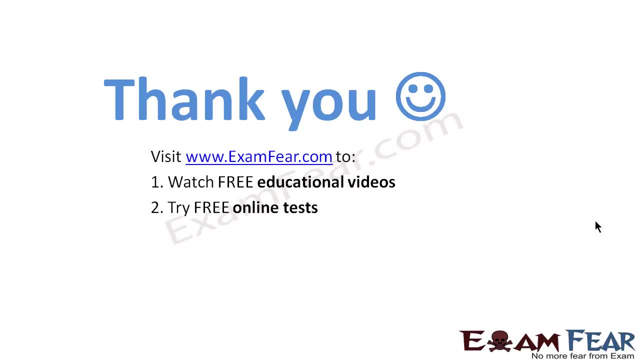 will say, for every two positive number, the sum is positive. thank you, visit examfearcom to watch free educational videos, try free online tests, get the best quality study materials, study from the best tutors and mentors, and much more. thanks once again. 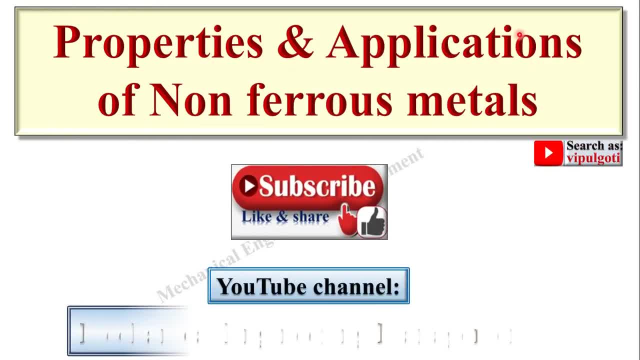 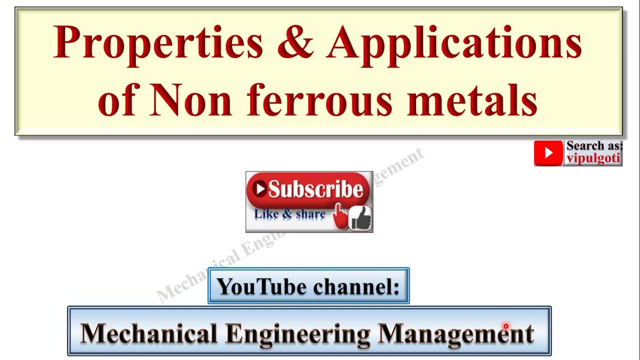 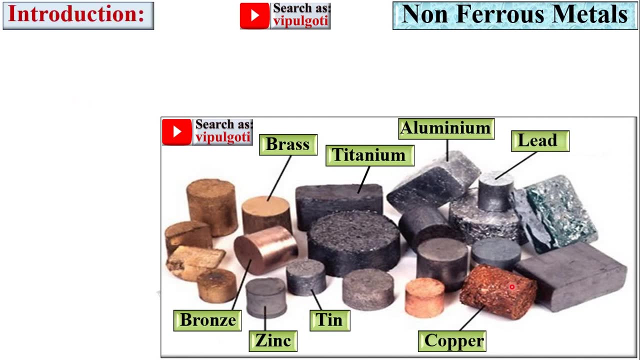 Today I am going to discuss about properties and application of non-ferrous metals. So welcome to my youtube channel, mechanical engineering management- Like, share and subscribe. Here you can see there are the different metals in which you can see: titanium, aluminium, lead, zinc, tin, copper. 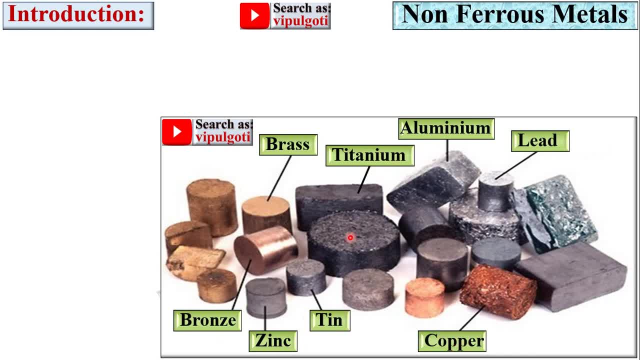 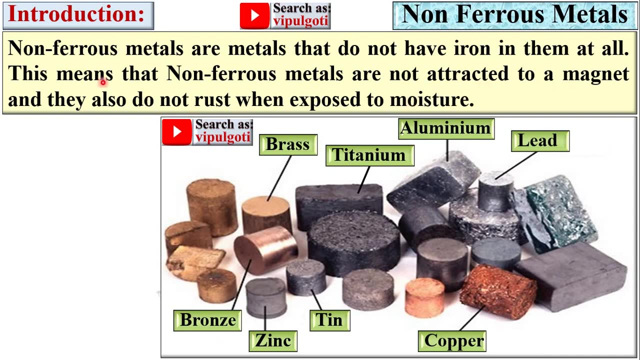 So these are the non-ferrous metals. So non-ferrous metals are metals that do not have iron in them at all. This means that non-ferrous metals are not attracted to a magnet because of there is no any iron in the non-ferrous metals, and they also do not rust when exposed to moisture.